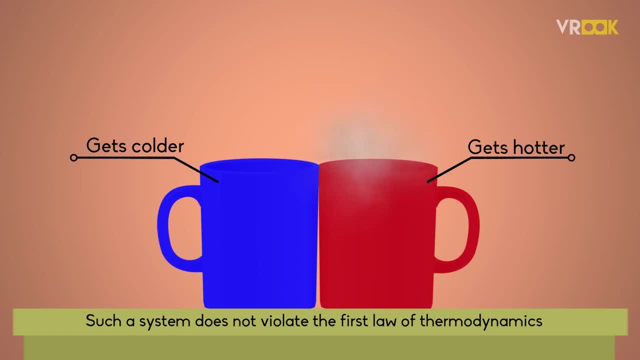 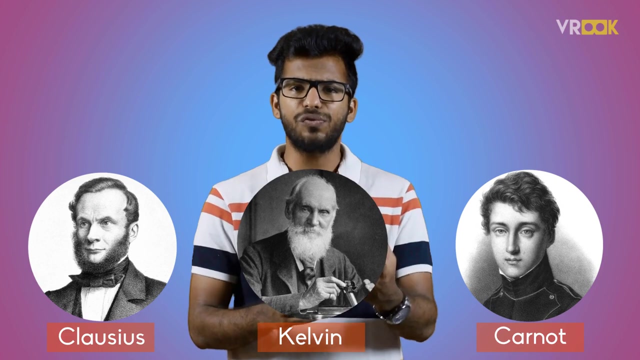 Obviously, we don't encounter such a system in nature. So to explain this and similar observation, physicists proposed a second law of thermodynamics. Clausius, Kelvin and Carnot proposed various forms of the second law to describe the particular physics problem that each was studying. 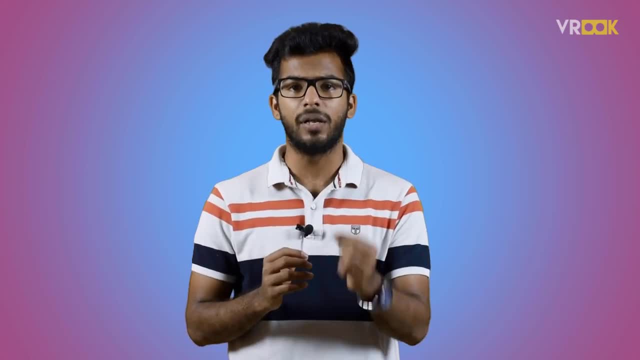 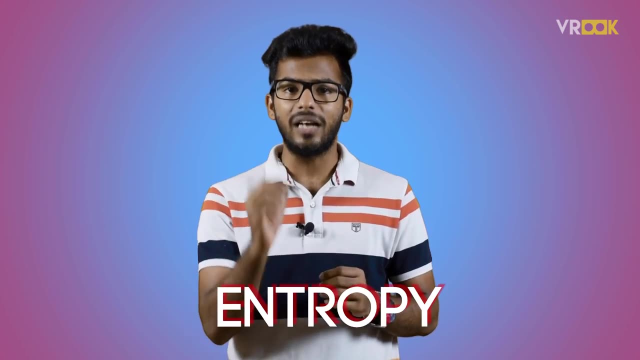 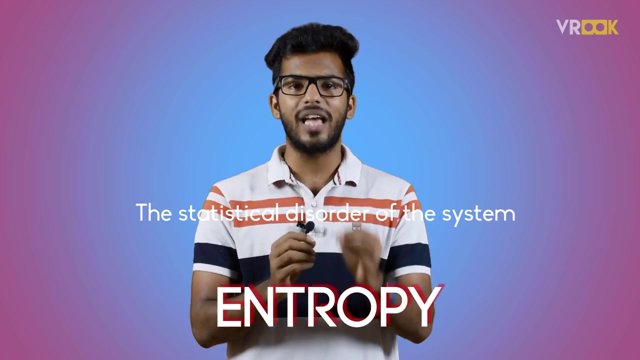 It begins with the definition of a new state variable called entropy. Entropy has a variety of physical interpretations, including the statistical disorder of the system, But for our purposes let us consider entropy to be just another property of a system, like enthalpy or temperature. 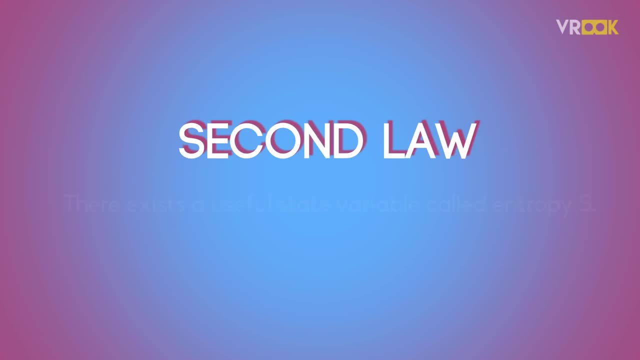 The second law states that there exists a useful state variable called entropy s. The change in entropy delta s is equal to the heat transfer of heat to the cold object. The change in entropy delta s is equal to the heat transfer of heat to the cold object. 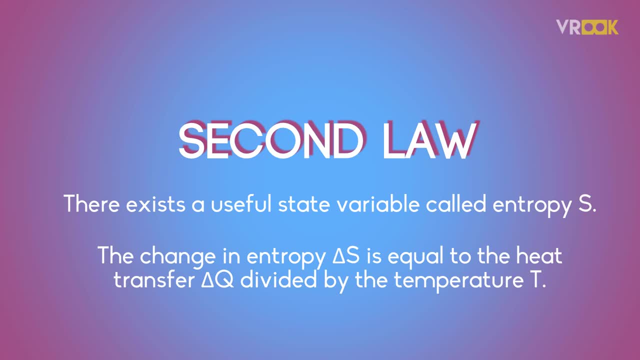 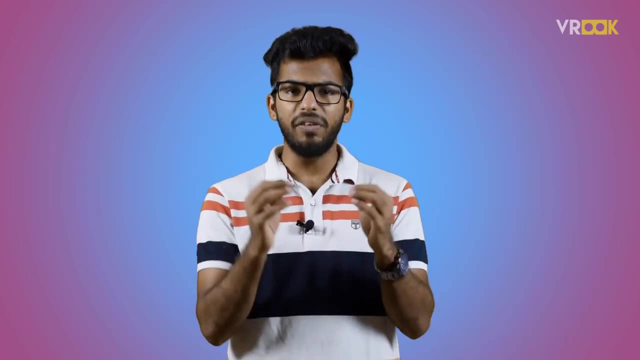 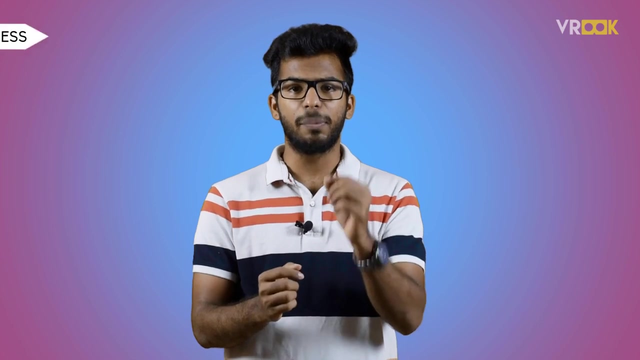 The version where heat is transferred is called Morun trzymeí. Heat transfer delta q divided by the temperature T For a given physical process, the combined entropy of the system and the environment remains constant if the process can be reversed. If we denote the initial and final states of the system by I and F, 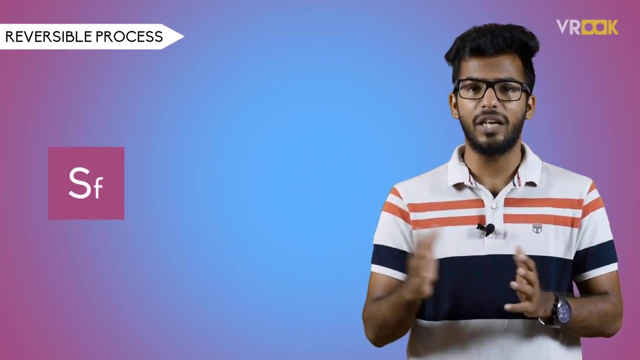 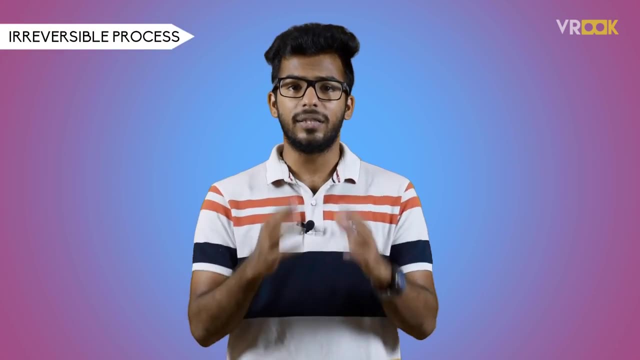 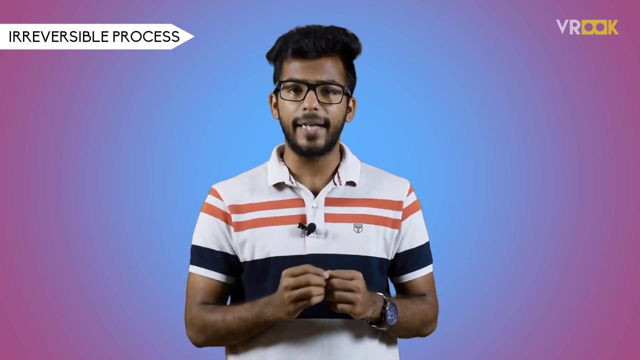 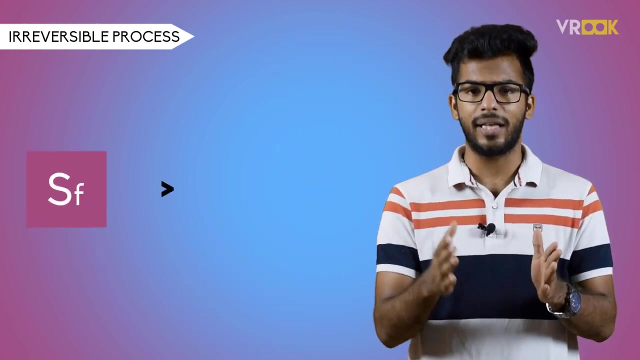 it should be: Sf is equal to Si. it should be S future, as f is equal to Si. The second law states that if the physical process is irreversible, the combined entropy of the system and the environment must increase. The final entropy must be greater than the initial entropy for an irreversible process, ie Sf greater than Si. 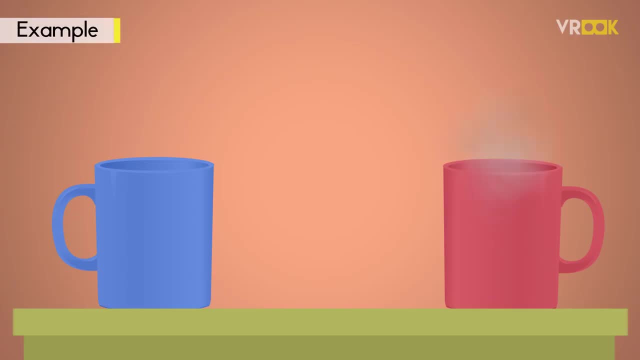 An example of an irreversible process is the problem discussed earlier in this video. A hot object is put in contact with a cold object. Eventually, they both achieve the same equilibrium temperature. If we then separate the objects, they remain at the equilibrium temperature and do not naturally return to their original temperatures.